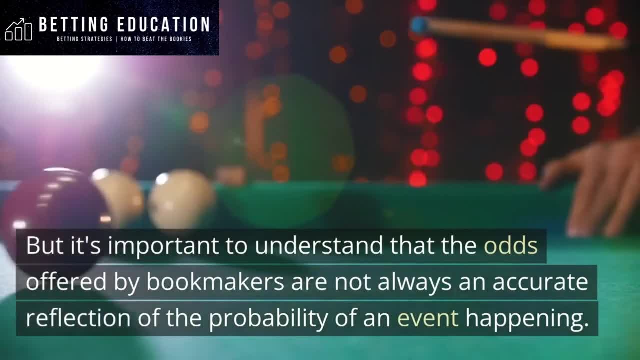 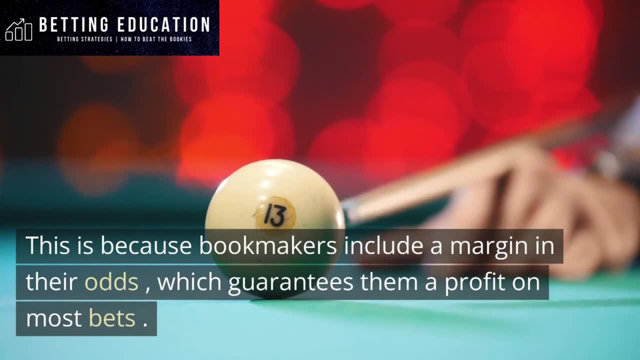 it's important to know that the probability of a team winning a game is 0.5, because if the odds offered by bookmakers are not always an accurate reflection of the probability of an event happening, This is because bookmakers include a margin in their odds which guarantees them a 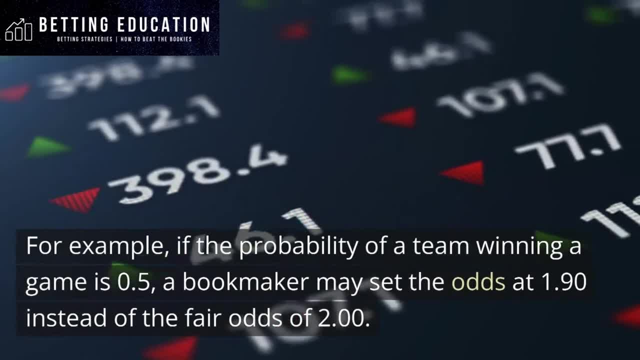 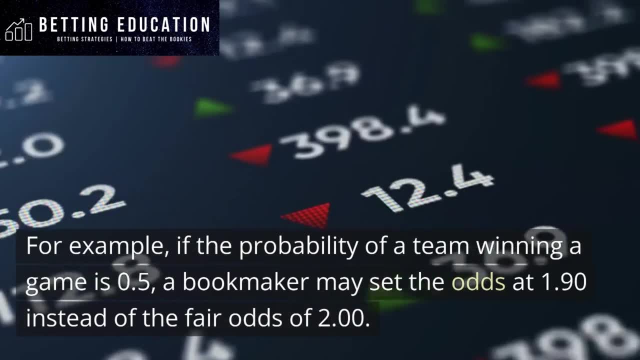 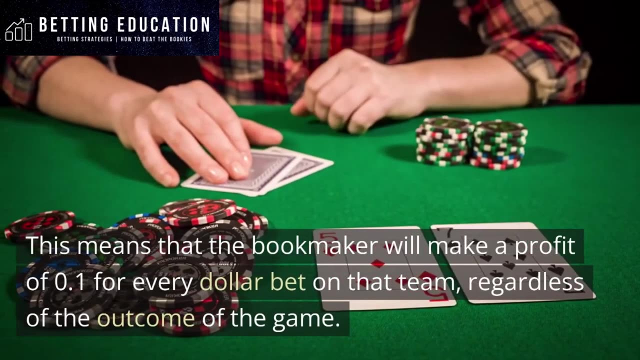 profit on most bets. For example, if the probability of a team winning a game is 0.5, a bookmaker may set the odds at 1.90 instead of the fair odds of 2.00.. This means that the bookmaker will make a profit of 0.1 for every dollar bet on that team, regardless of the 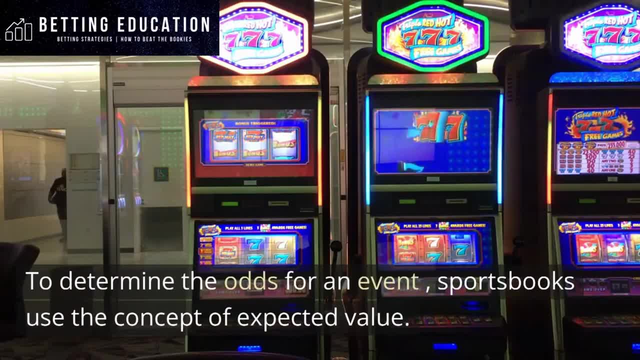 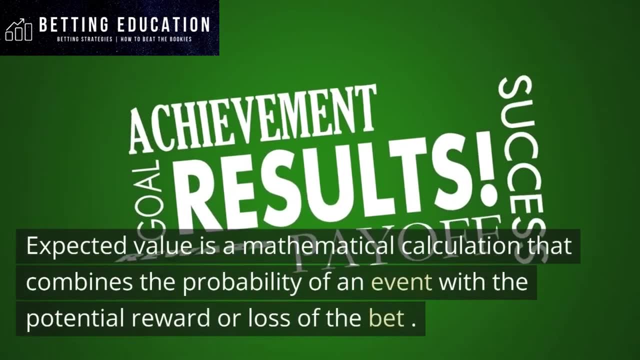 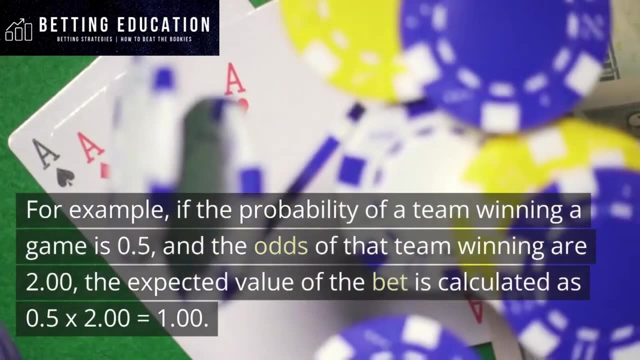 outcome of the game. To determine the odds for an event, sports books use the concept of expected value. Expected value is a mathematical calculation that combines the probability of an event with the potential reward or loss of the bet. For example, if the probability of a team winning a game is 0.5,. 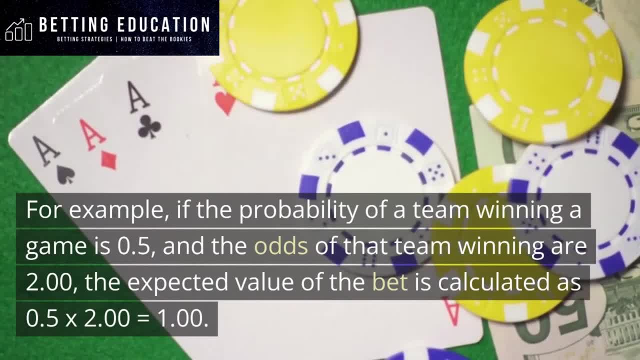 and the odds of that team winning are 2.00,. the expected value of the bet is calculated as 0.5 x 2.00 equals 1.00.. If the probability of a team winning a game is 0.5, and the odds of that team winning are 2.00,. 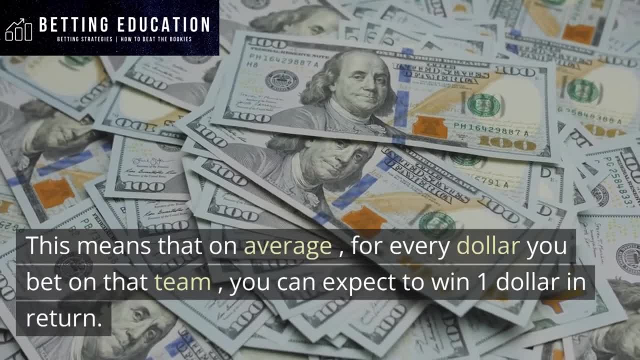 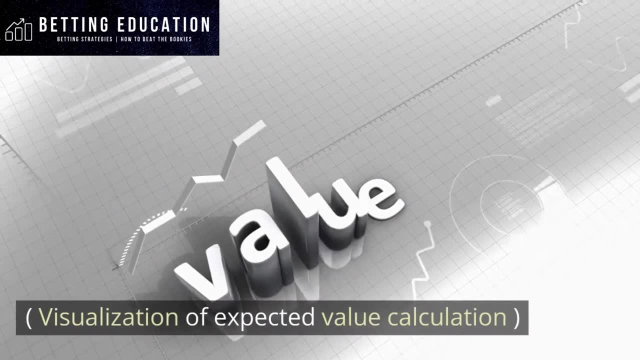 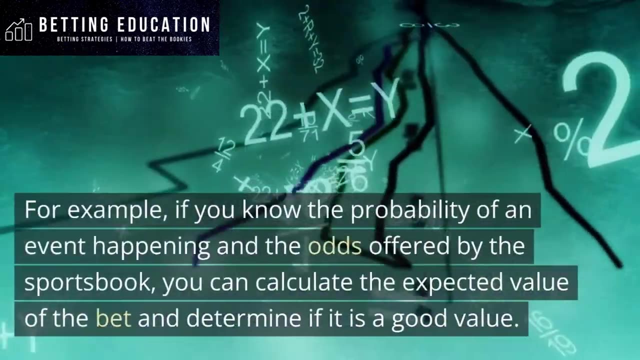 this means that on average, for every dollar you bet on that team, you can expect to win $1 in return. Visualization of Expected Value Calculation. By understanding the math behind sports betting, you can make more informed and intelligent bets. For example, if you know the probability of an. 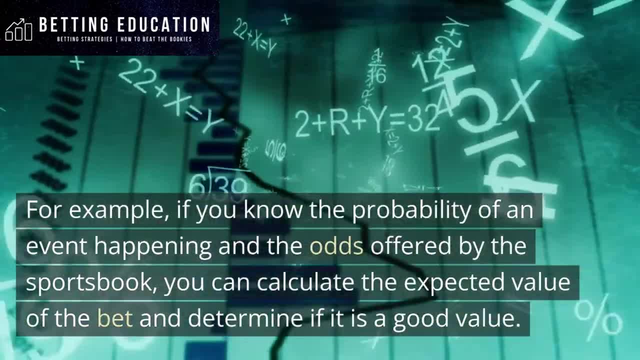 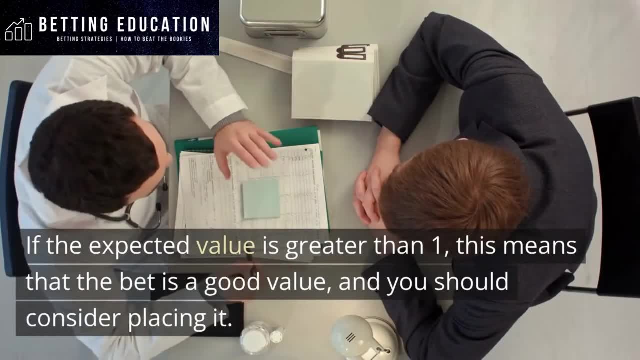 event happening and the odds offered by the sports book, you can calculate the expected value of the bet and determine if it is a good value. If the expected value is greater than 1,, this means that the bet is a good value and you should consider placing it. 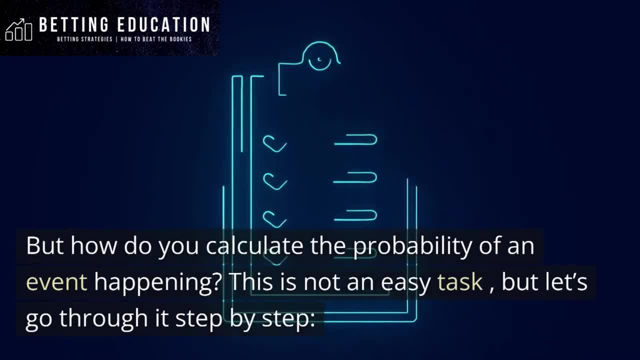 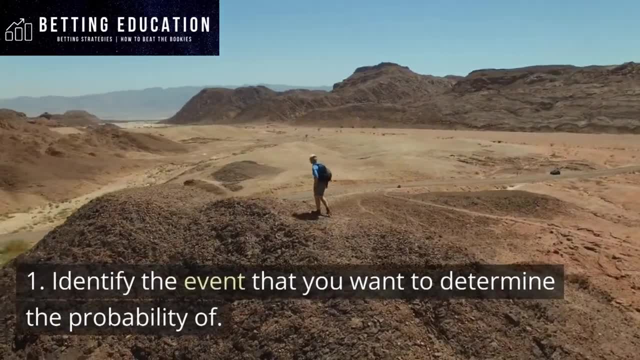 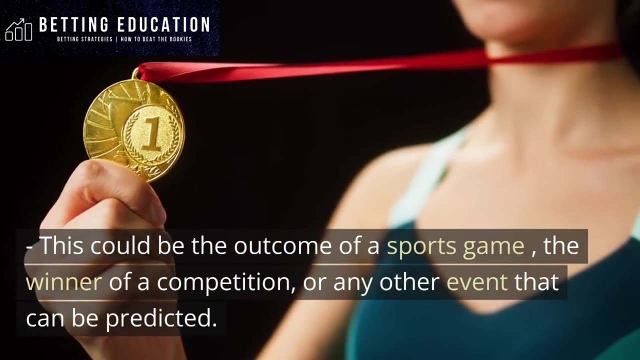 But how do you calculate the probability of an event happening? This is not an easy task, but let's go through it step by step. 1. Identify the event that you want to determine the probability of. This could be the outcome of a sports game, the winner of a competition or any other event that can be predicted. 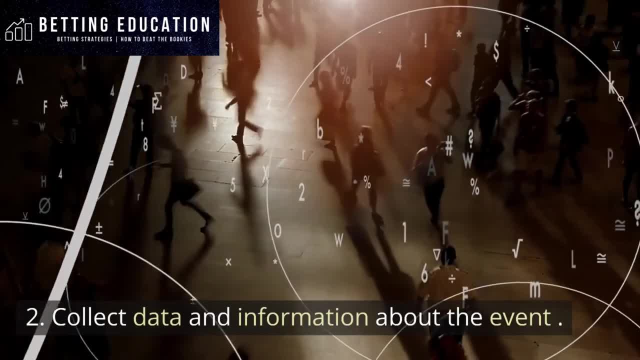 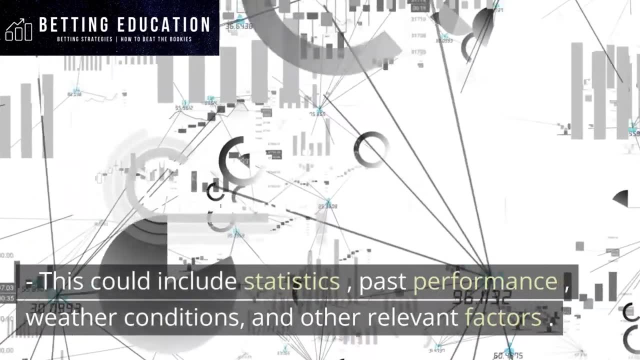 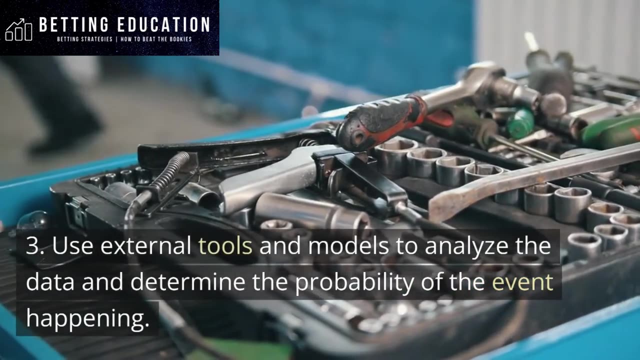 2. Collect data and information about the event. This could include statistics, past performance, weather conditions and other relevant factors. 3. Use external tools and models to analyze the data and determine the probability of the event happening. This could include statistical. 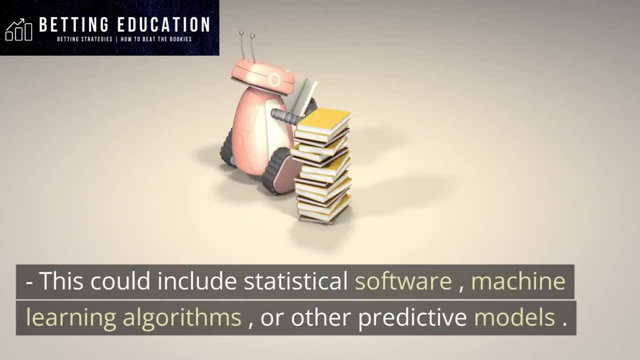 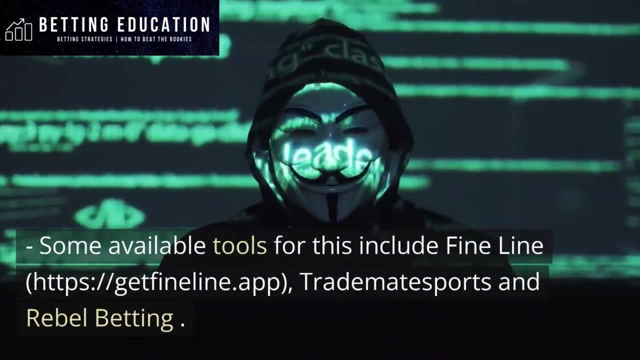 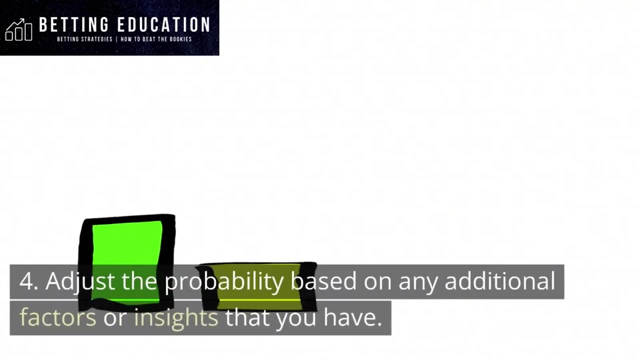 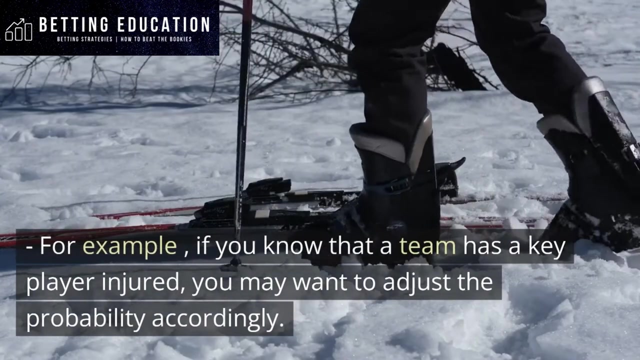 software, machine learning algorithms or other predictive models. Some available tools for this include Fineline, Trademate Sports and Rebel Betting. 4. Adjust the probability based on any additional factors or insights that you have. For example, if you know that a team has a key player injured, you may want to adjust the probability accordingly. 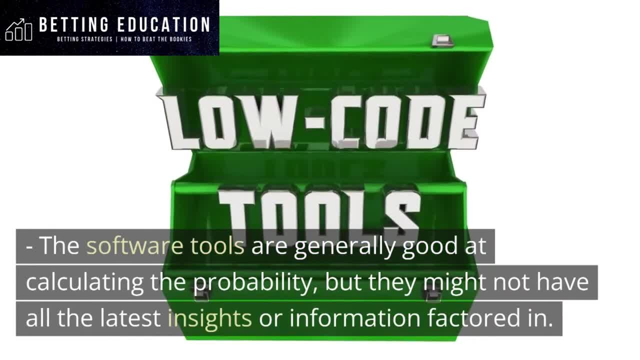 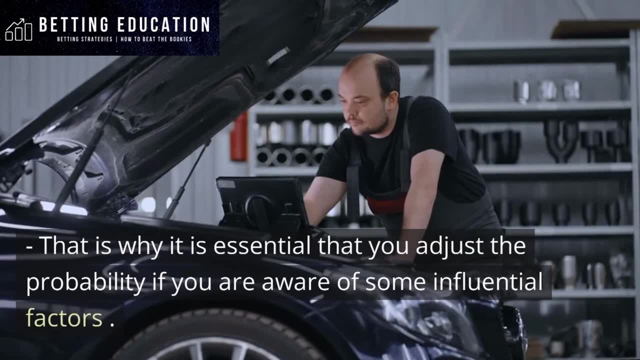 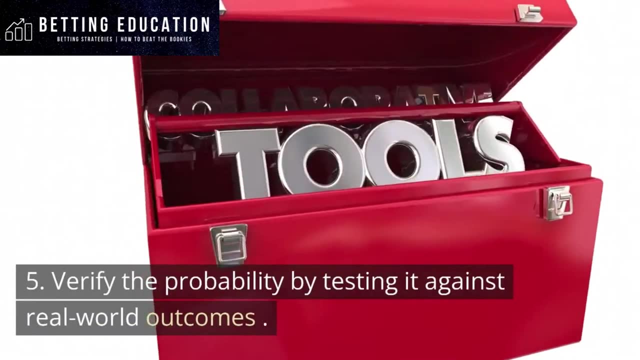 The software tools are generally good at calculating the probability, but they might not have all the latest insights or information factored in. That is why it is essential that you adjust the probability if you are aware of some influential factors. 5. Verify the probability by testing it against real-world outcomes. 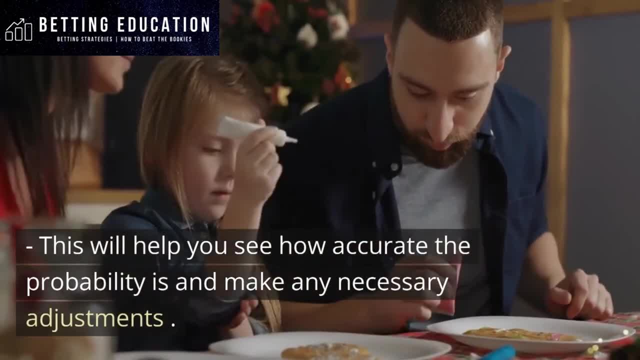 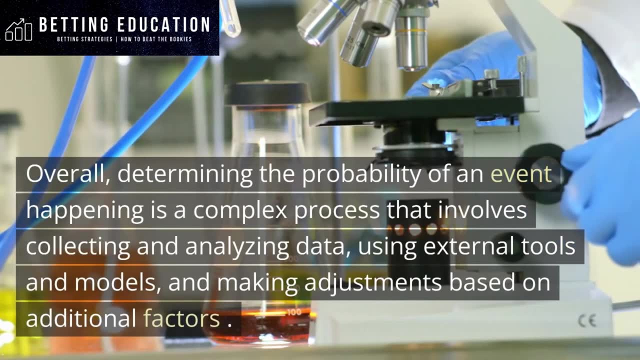 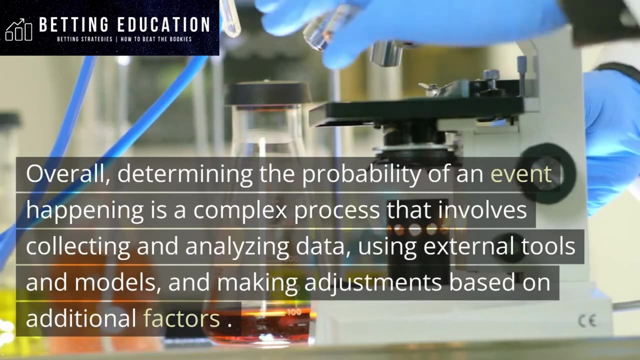 This will help you see how accurate the probability is and make any necessary adjustments. Overall, determining the probability of an event happening is a complex process that involves collecting and analyzing data using external tools and models and making adjustments based on additional factors By following these steps and using the right tools and models. 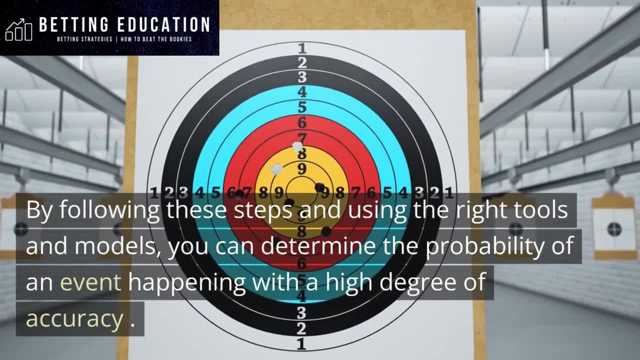 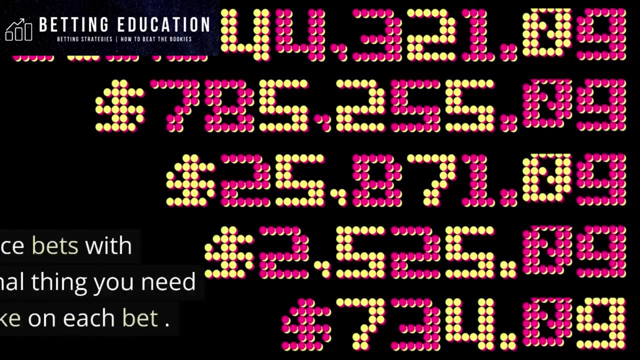 you can determine the probability of an event happening with a high degree of accuracy. When you know the probability of an event, it is easy to calculate the expected value for the bet. All you have to do now is to place bets with expected value above 1.. 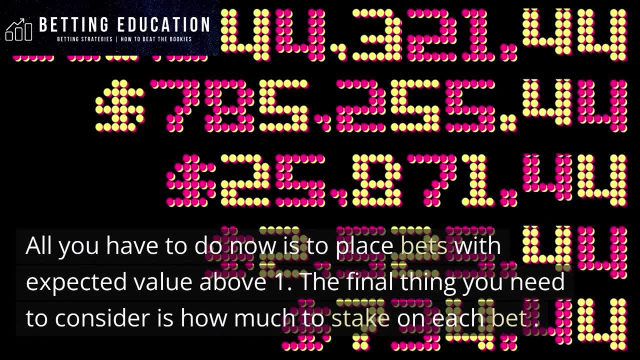 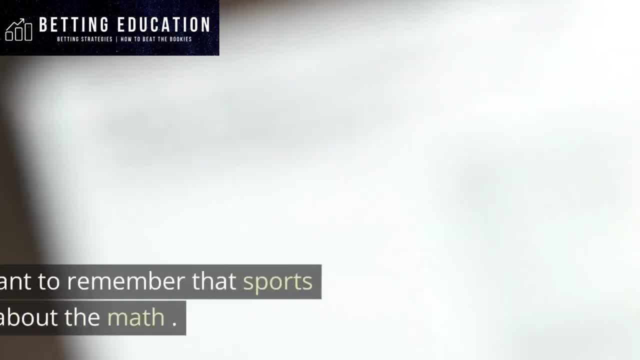 The final thing you need to consider is how much to stake on each bet. There are many different staking plans, and we made another video explaining these. Be sure to check it out. Lastly, it's important to remember that sports betting is not just about the math. 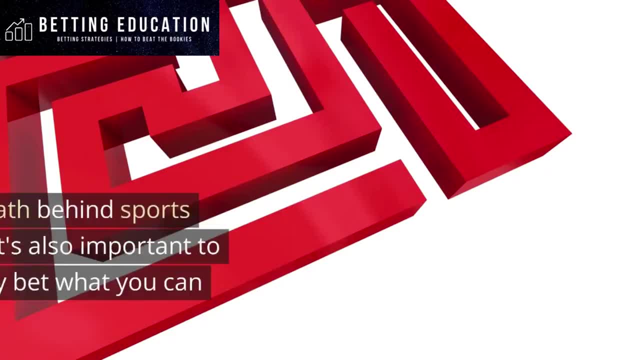 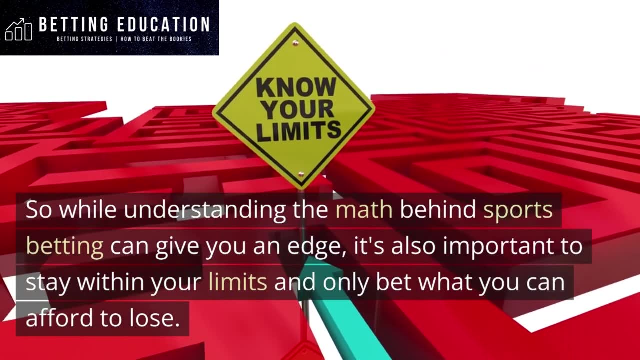 It's also about having fun and enjoying the thrill of the game. So, while understanding the math behind sports betting can give you an edge, it's also important to stay within your limits and only bet what you can afford to lose. We hope you enjoyed our video on the math behind sports betting and found it informative and helpful. 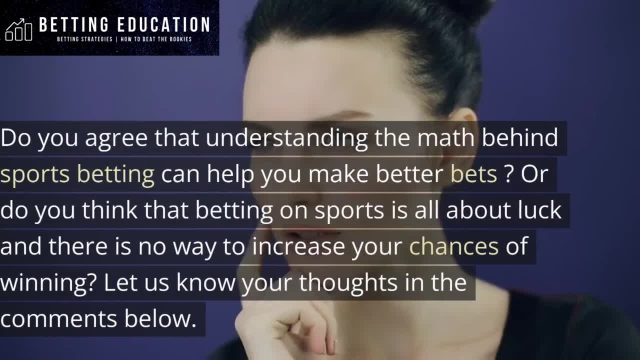 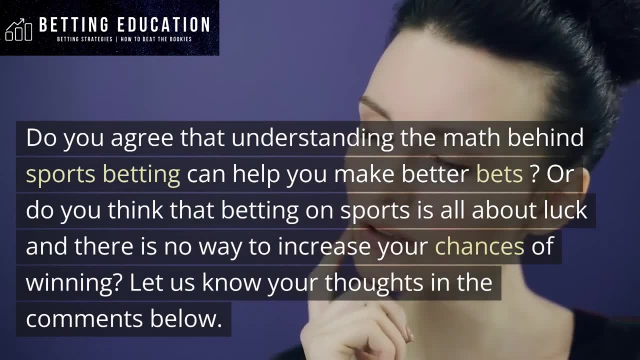 Now we want to hear from you: Do you agree that understanding the math behind sports betting can help you make better bets, Or do you think that betting on sports is all about luck and there is no way to increase your odds? Do you think that betting on sports can increase your chances of winning?